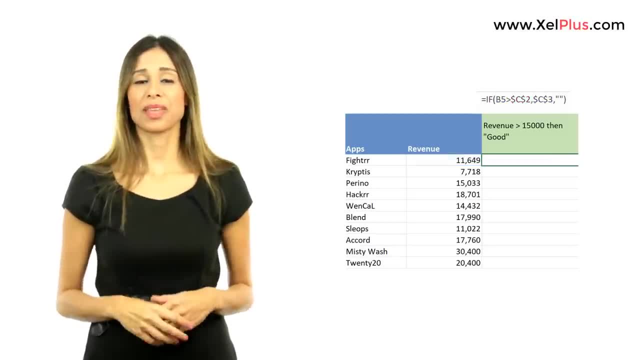 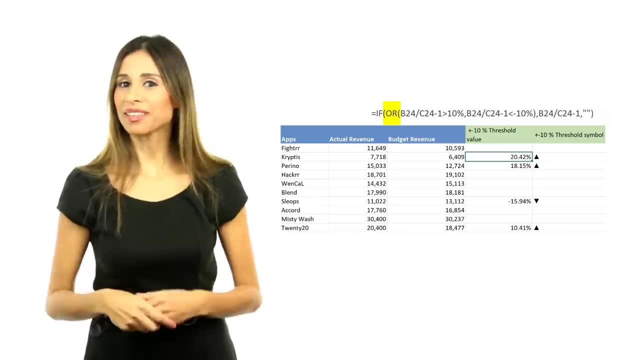 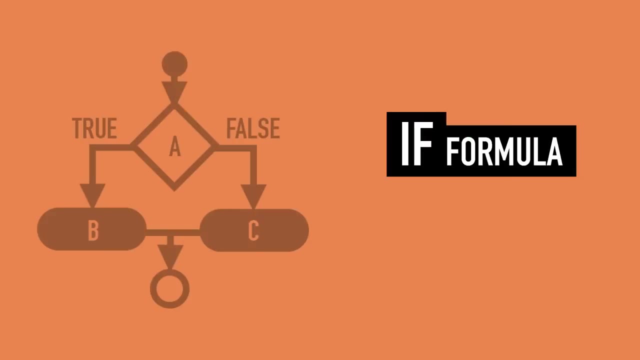 Today's video is about Excel's if function. How can we use it alone, How do we know if we need more than one if, And how can we combine it with other logical functions, such as and or or functions- Whenever you need a formula that's based on a condition. 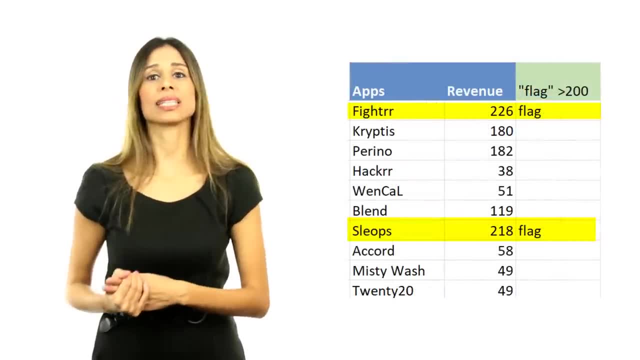 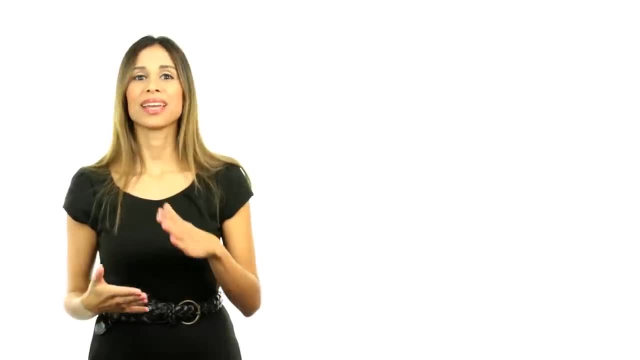 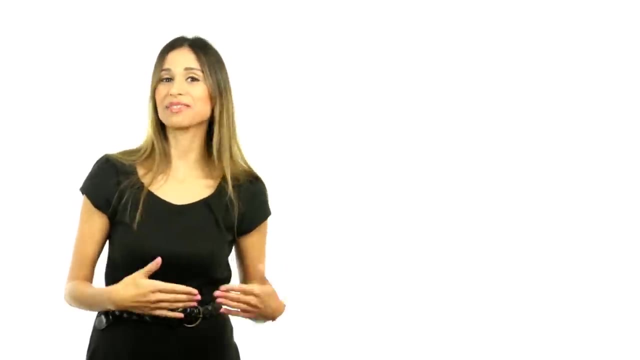 such as you need to mark or flag entities separately if their value is above 200 in revenue. an if can do a good job here. Now the way you know if you need a nested if that means you need to use another if inside an if. 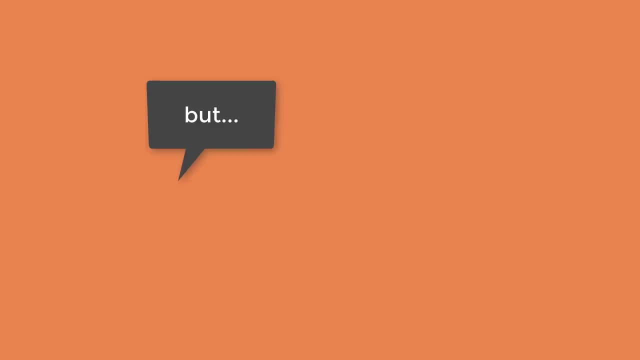 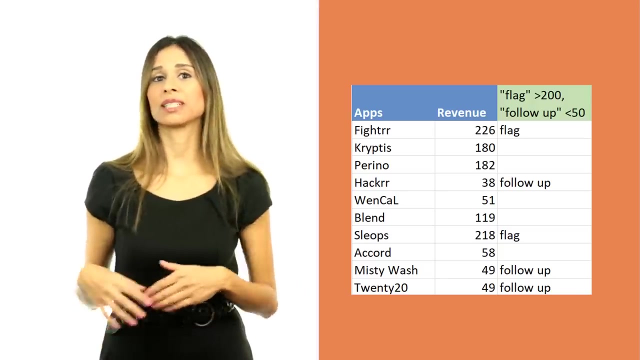 is when you use buts in your sentences. So let's say, we need to mark entities if their value is above 200, but if their value is below 50, we need to follow up on them. Let's take a look at some examples. 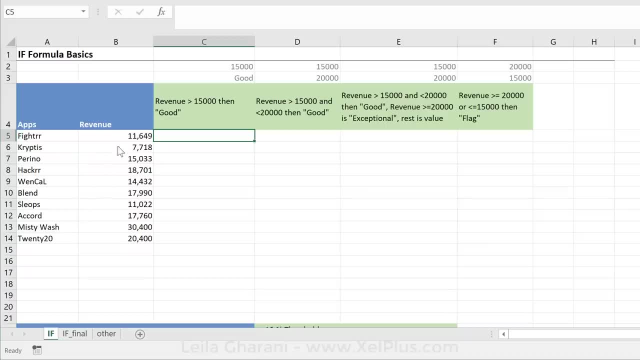 In this example, I have a list of apps and I have the revenue that's associated with each app. Now I've been asked to solve for these. For the first case, I need to mark apps with the word good if the revenue is above 15,000. 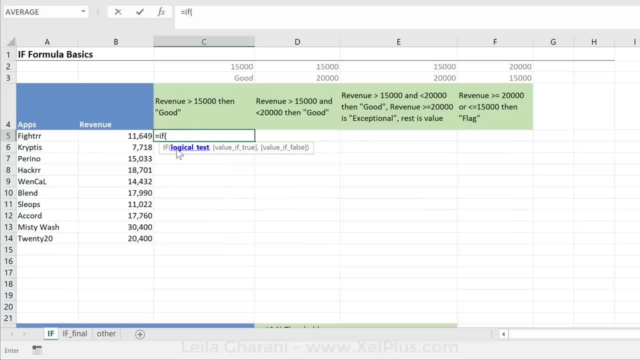 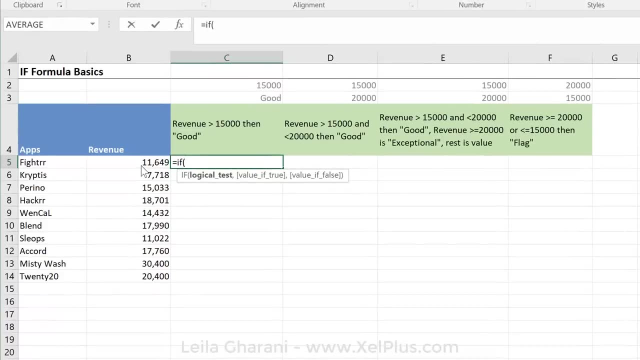 So we're going to start off with: if The first argument is our logical test, What is our logical test in this case? Is this value right? That's our revenue, and if this is greater than 15,000,. so I can either type it in like this: 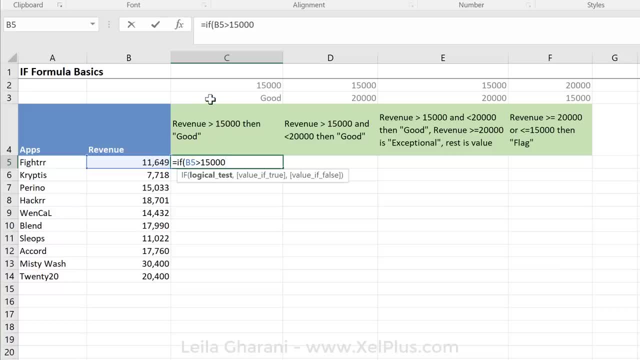 or if I have these values in other cells, I can reference those cells And obviously you're going to be more flexible if you go with the cell referencing route, because it could be that I change the threshold next month to 20,000.. 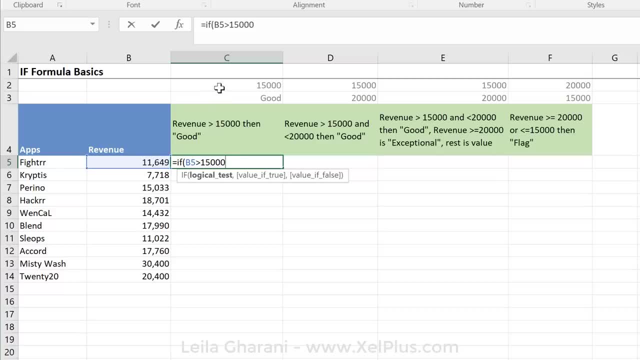 And it's much more transparent and easier for me to manage if I just have to go to one cell and change that number, instead of finding the formula, changing it in that formula and then dragging it down and making sure that it applies to everything else. 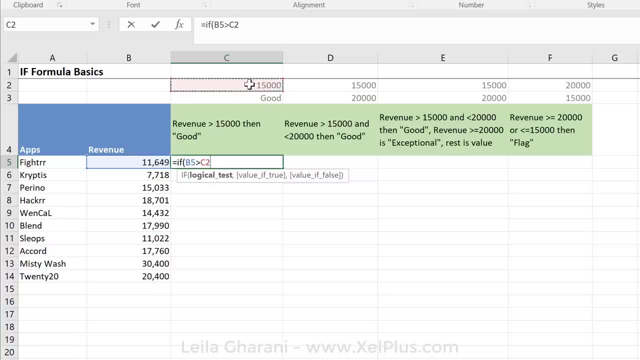 I'm not going to type it in here, I'm actually going to reference this cell. but when you do the cell referencing route you have to keep the fixing in mind, right, And that I can do in one go with the F4 key. 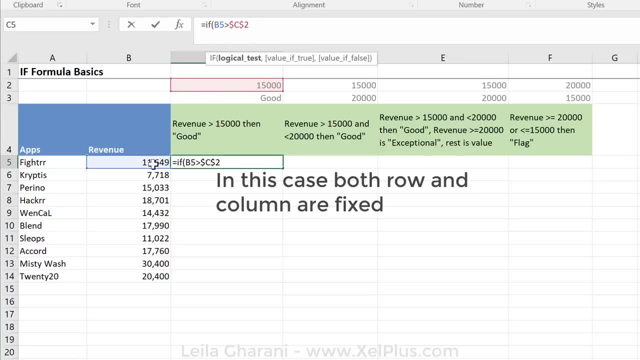 That's basically my logical test Check. is this value greater than this value? If it is, then we go to our next task argument. what should it do now? here I want to type in good and again. I can type it in like this, but you have to be careful, because if you're typing text in 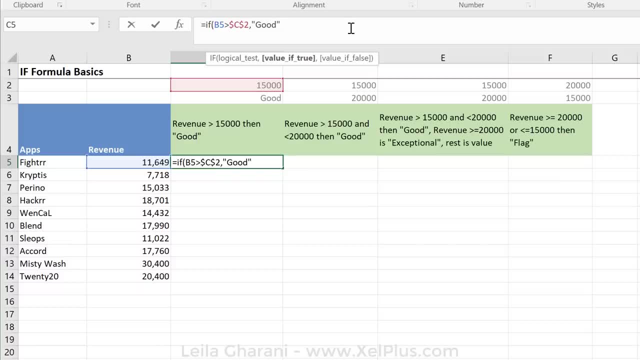 a formula, you have to put it in quotation marks. in this case, I also want to do a cell reference. so I'm going to reference this cell and, again, I'm going to fix it. okay, so that's what it should do if this does happen and if it doesn't. 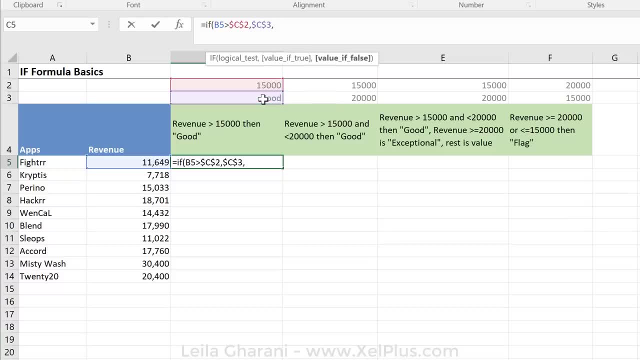 happen, then I want it to do nothing, and nothing in Excel means you can put in a double quotation mark, close the bracket, press Enter. now we're going to send this formula down and just double check. this is about 15,000 and these are above 15,000. okay, so it looks good. now let's go to the next one. it's not just about 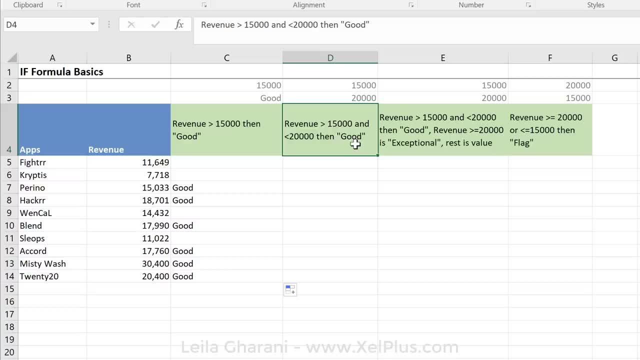 15,000, but we want to mark the entities as good if the revenue is greater than 15,000 and less than 20,000. okay, so situations like this call for the and function inside the if function and allows us to do a logical test for more than one thing, and in this case we have two. 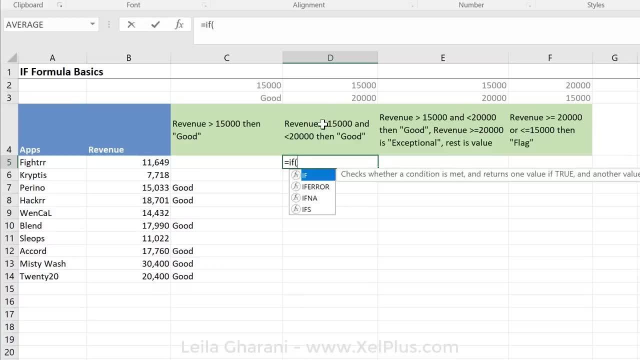 things to check for. so we're still going to start off with our if, but right here, before we start typing in our logical test, we are going to put the AND function first and type in all our tests that should occur and should be true inside the AND function. 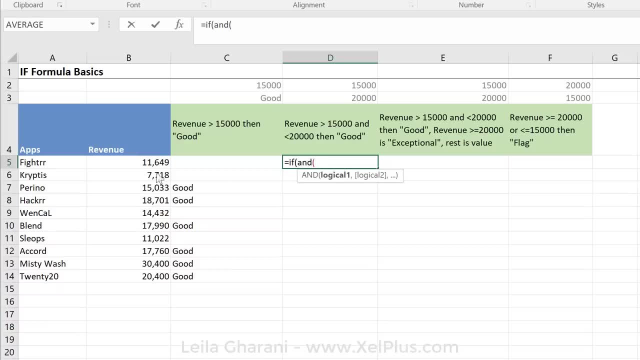 Okay. so what's one of these logical tests? It's the same one we had before, so is this revenue value greater than this value? And I'm going to fix it. The next argument is your second logical test, And that's again: is this value? 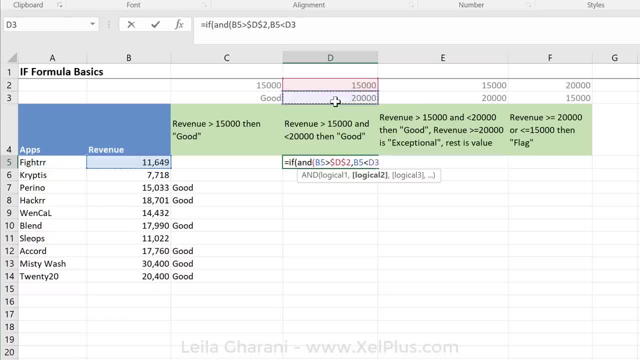 now we want to say: is it less than this value? and I'm going to fix it as well. Now, don't forget to close the bracket for the logical test, so for our AND condition here. Then the next argument is: what should it do? 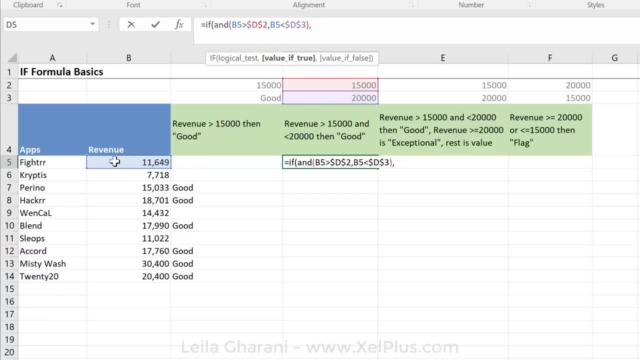 if both of these occur, So if revenue is in between 15,000 and 20,000.. Well, we said we want good. in this case I'm going to type it in. Otherwise we want nothing. Close the bracket. 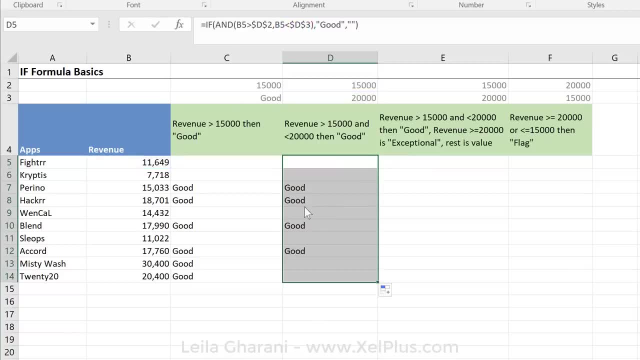 Press enter. Let's see if it filters it out correctly. So these are between, this is between, and that's between. these are too high. Next challenge: If revenue is greater than 15,000 and 20,000, so this is similar to what we did before. 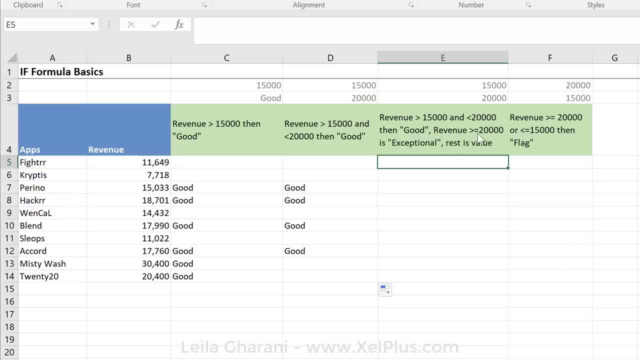 but now we have an additional condition: If revenue is greater than or equal to 20,000, we want them marked as exceptional, And rest is value. By value I mean just the value that's in the cell. So basically, we're going to have a mixed column. 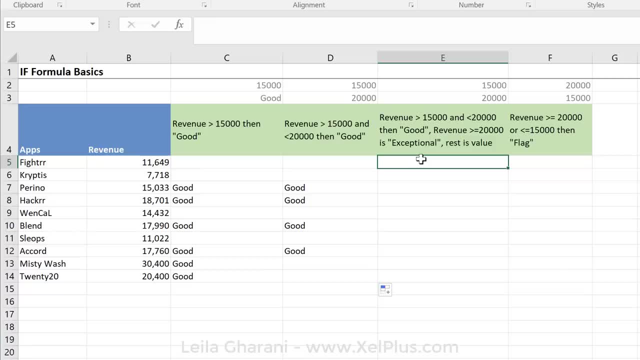 some text and some numbers in here. How do we deal with these conditions? Well, the first part is exactly like we did before, So I'm actually going to copy this, just press escape to leave and paste it in here. Let's just bring in my cell references up here. 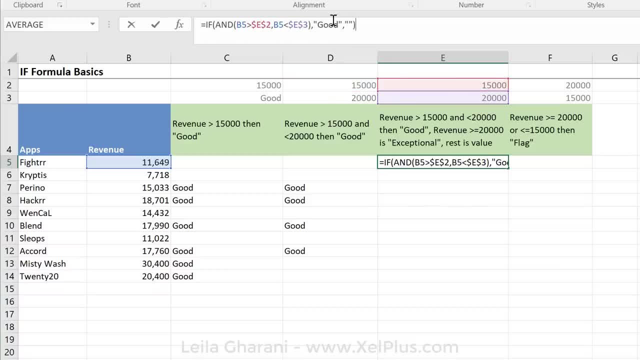 Okay, if both of these conditions occurs, then I want good. Otherwise, do I want nothing now. No, because I'm not done with the formula. I need to test for another condition. So if this doesn't happen, I still now need to go and test. 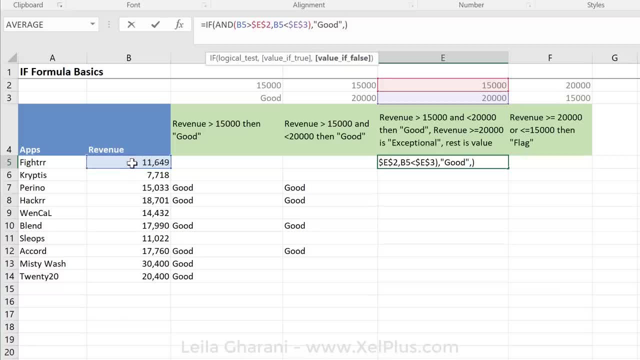 is this app an exceptional app in terms of revenue. So exactly in the value. if false argument, that's where you need to put your second if condition. What is our logical test? This number Now, is it greater than or equal to this number? 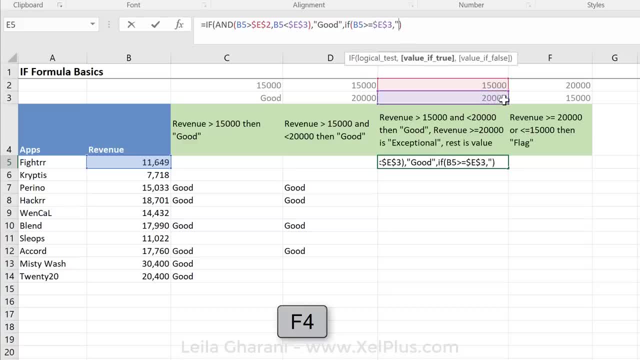 Now I'm going to fix this. Then, what do we want? We want it to write exceptional, Otherwise otherwise means, if none of these occurred until now, what should it do? We said we want the value, so I'm just going to do a cell reference here. 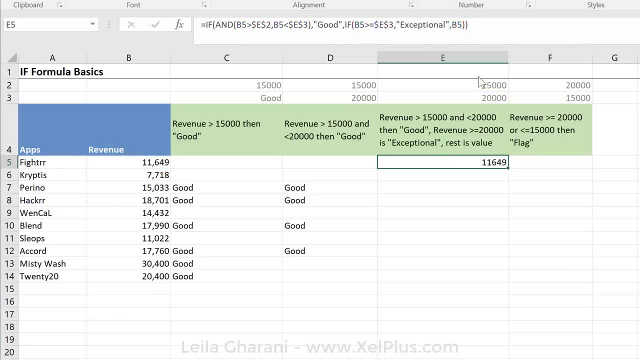 And now I have two. I have two ifs, so I need two brackets. Let's just send this down. So now we have the good, we have the exceptional and for everything else we have the number. Okay, so that's how you can use nested ifs in your formulas. 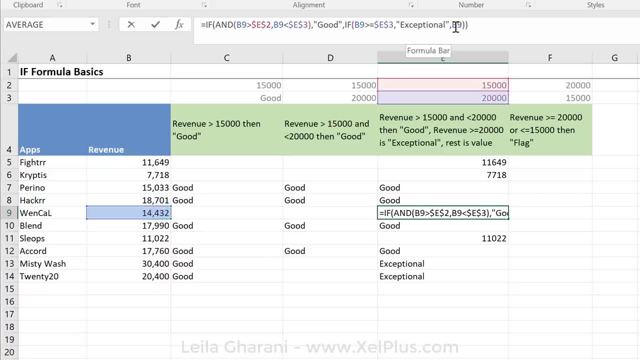 And you're not restricted to two ifs. You can obviously put another if here. If the value is below another threshold, then do this. Otherwise, put something else, Put the value or put nothing. It's just that the more nested ifs you have, 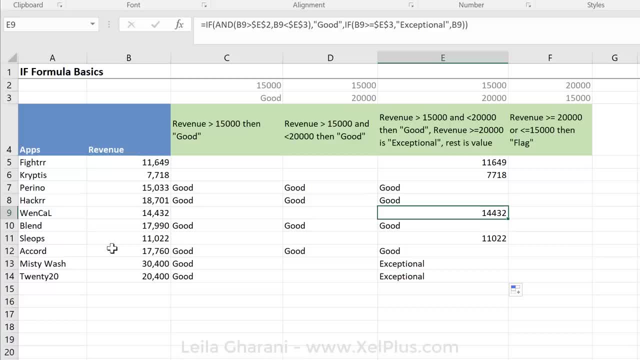 the more difficult it's going to get to understand the formula. One thing to keep in mind is that Excel does leave the formula the moment it comes across a true condition. So the moment this is true, it puts back good and it leaves the formula. 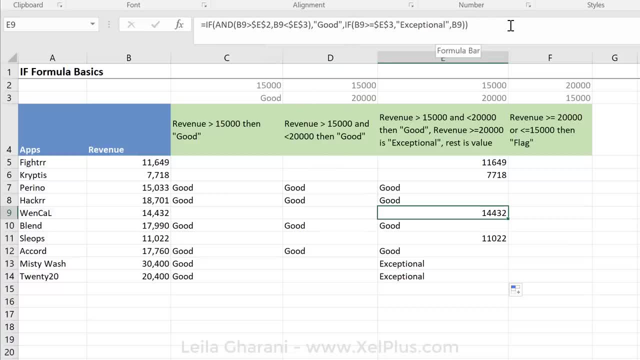 It doesn't go and evaluate all your other if conditions. So that's something to keep in mind when you're writing these more complex formulas. Now let's look at the next one. Let's look at another case. If revenue is greater than or equal to 20,000. 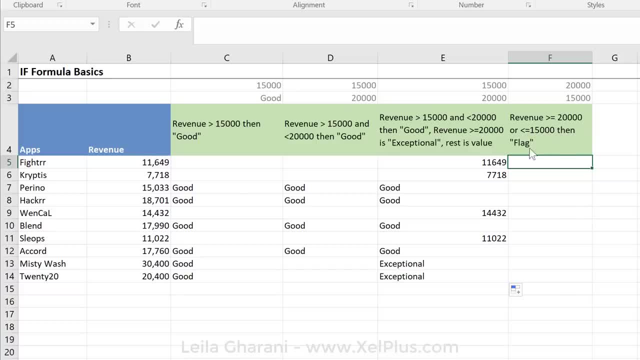 or it's less than or equal to 15,000, then we want to type in flag. So, basically, anything in between we're going to leave alone. How do we write this? I'm going to start with the if. Now, another logical test that we can use is the or function. 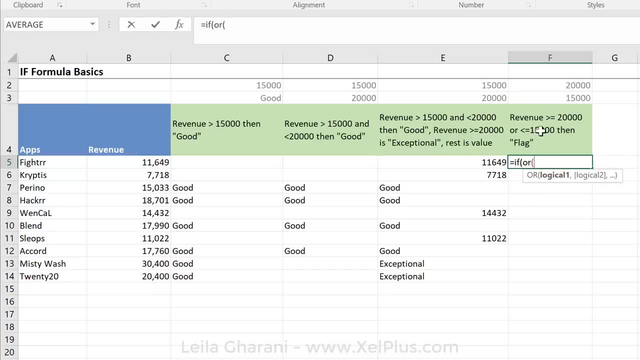 An or checks for if either of these conditions apply. So the logical test one: is this one greater than or equal to this number? We're going to fix it. What is logical test two? Is this number less than or equal to this number? 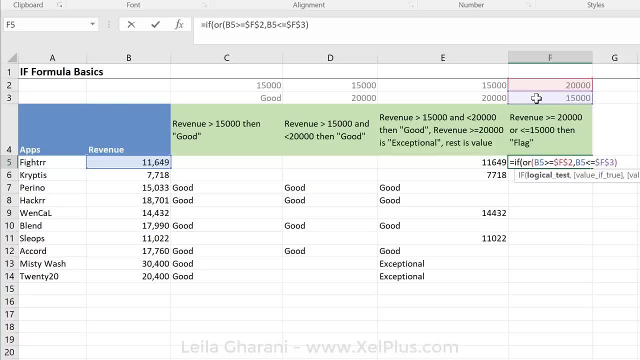 And we're going to fix it. And don't forget to close your or condition before you leave. So there's something I sometimes forget. I continue going and then I realize, oh, I forgot to close that condition. So next one: what should it do if either of these occur? 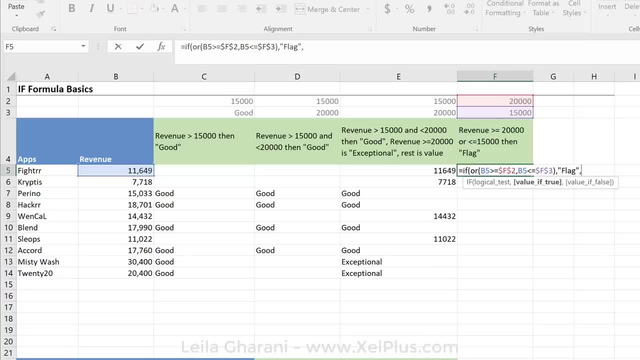 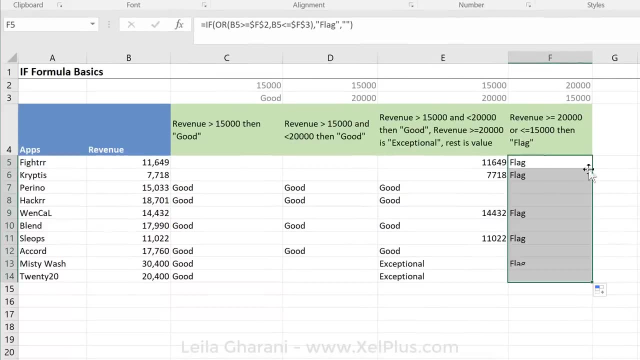 Well, we just want to type in the word flag there, Otherwise we're going to leave them alone and put nothing. Okay, so it flagged the first one. Let's see if that's correct. Is that less than Yes, because it's not in between these. 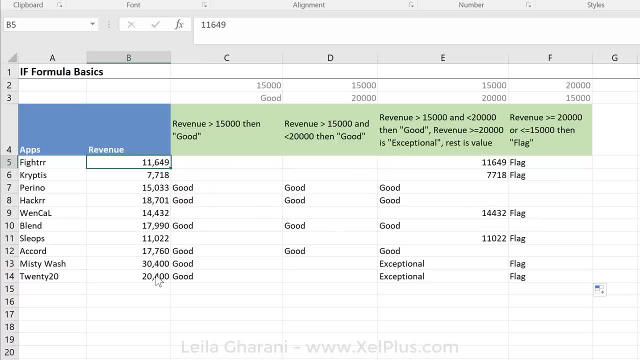 Flag these, these and these. Okay, so that looks good. Now let's take a look at another case where we're going to use bigger forms. where we're going to use bigger forms, where we're going to use bigger formulas. 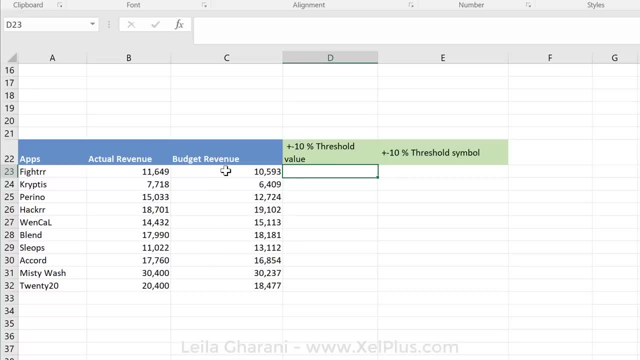 inside our logical test argument. We have budget values and we want to show the percentage difference. so basically show the deviation from actual to budget. if that deviation is a bigger deviation, that's plus or minus 10%. Whenever you come across cases where you have formulas inside your if function. 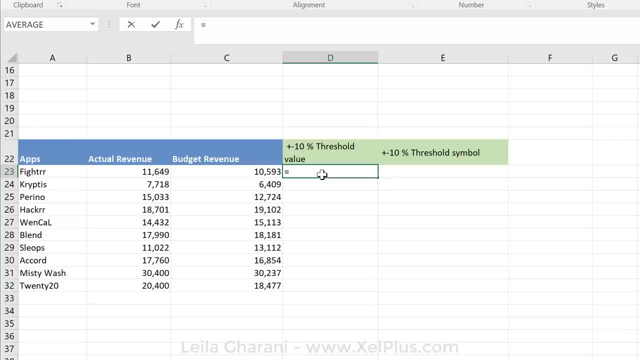 it's easier to start with the core formula first. The core formula in this case is my deviation, So I'm just going to calculate that actual divided by budget minus one. Let's just drag this down and see what we get. The aim is not to put anything for these ones. 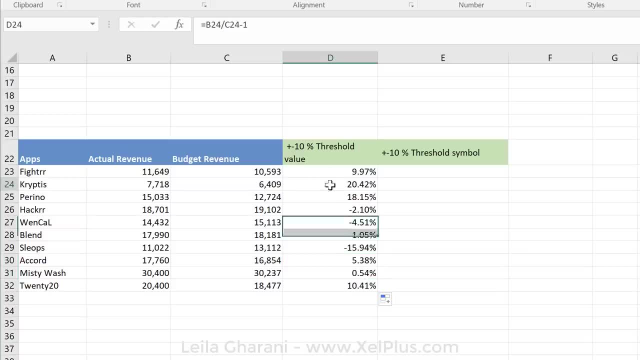 that are between plus or minus 10%. So only put in the bigger deviations in here, which actually is these four numbers. Okay, so how do we do that? Let's start off with this. Let's start off with our. if That's a part of my logical test, right? 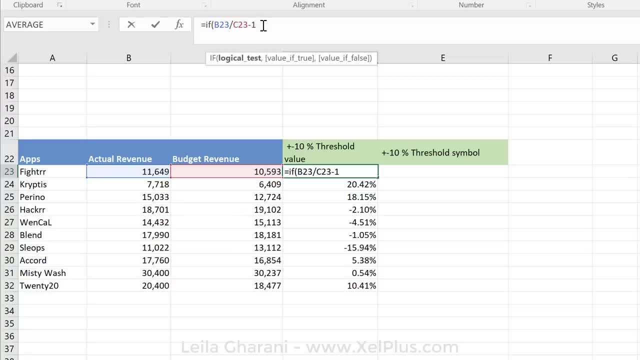 I want to evaluate the answer of this formula. What do I need to put in here? How do I handle that? I need the or function right, And the or always comes before, So right after the, if I'm going to type in the or. 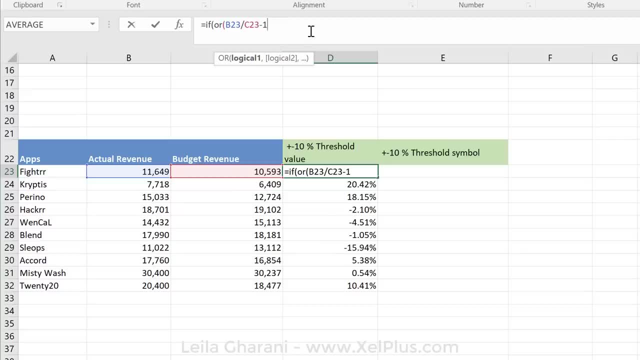 My logical test one is to check the results of this formula and see is it bigger than 10%. Okay, that's the first logical test. The second one is: take a look at the same formula and see is it less than minus 10%. 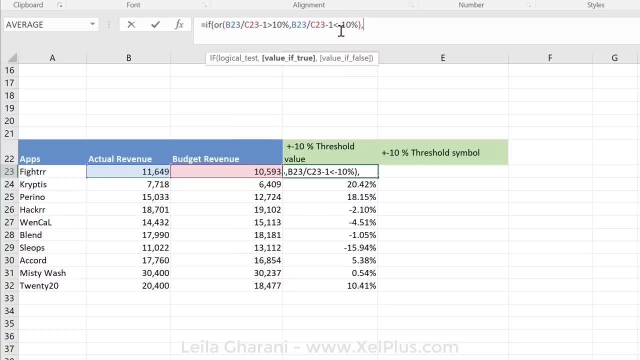 Okay, we're going to close the bracket for the or condition. What should it do if it's true? Well, it should give me back the deviation. So I'm going to paste that formula in there. Otherwise, it should leave it alone and do nothing. 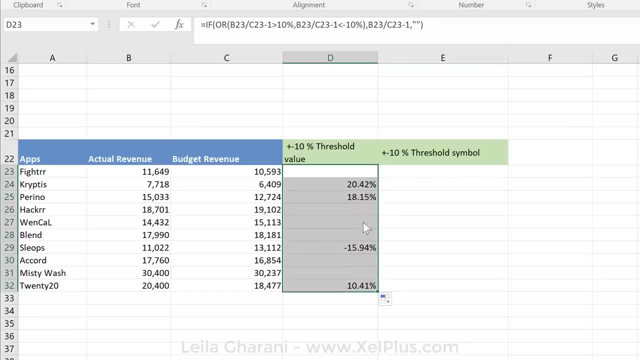 So I'm going to close the bracket And I should just get these four numbers. Okay, and in the last example here I just wanted to show you that you can also use symbols as your results. So let's say, for the positive deviations. 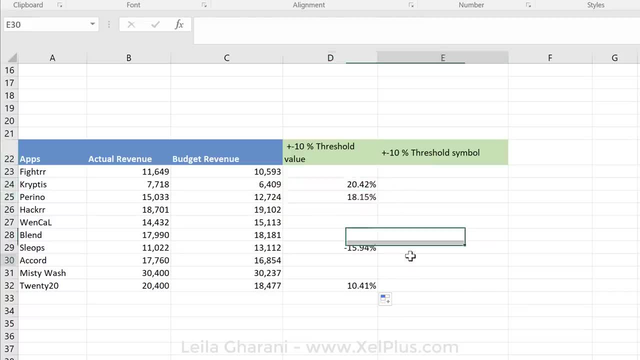 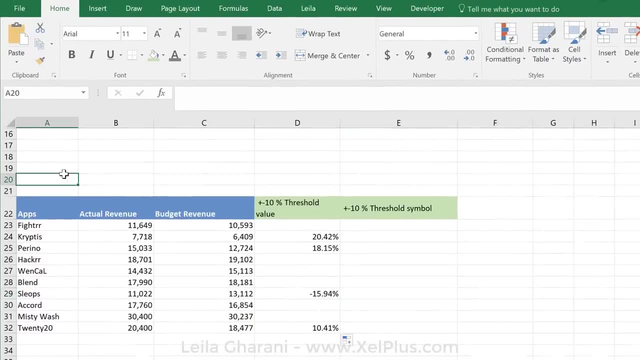 I wanted an up arrow And for the negative deviations, or the deviation in this case, I wanted a down arrow. First step is to bring your symbols in your Excel sheet, So I'm going to do that by going to Insert Symbols. 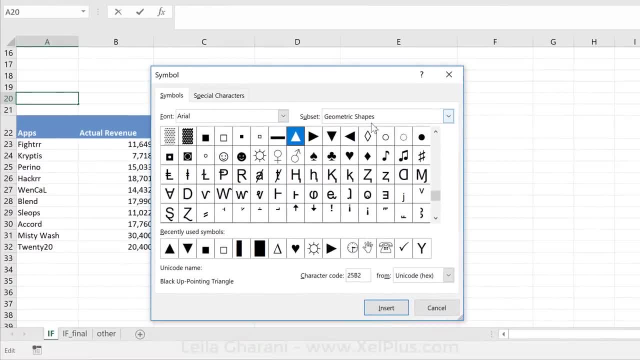 The symbols I use most often are under Arial Geometric Shapes And you can see them actually here. Just find the ones that you like and click on them, press Insert. So that's the up one and I want the down one. 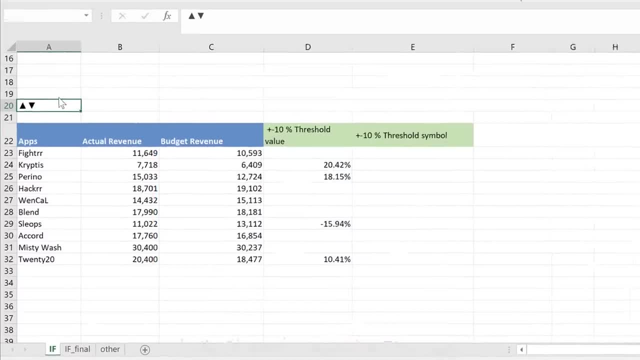 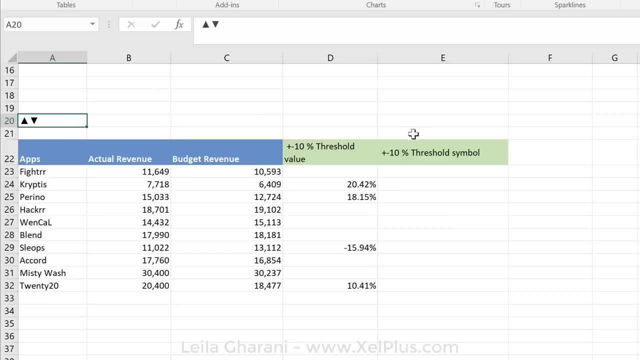 I'm going to press Insert right there and then Close. I can use them as text inside formulas by putting them in quotation marks, but I actually want to do cell references to them, So if I decide to change the symbol to something else, 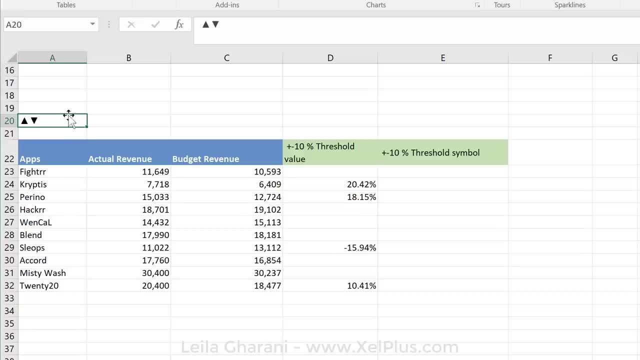 for another type of report. all I have to do is is replace that symbol in the cell. So I'm going to put them in two separate cells. So let's Control X, cut this one out and put it right here. Can I use the same formula for here? 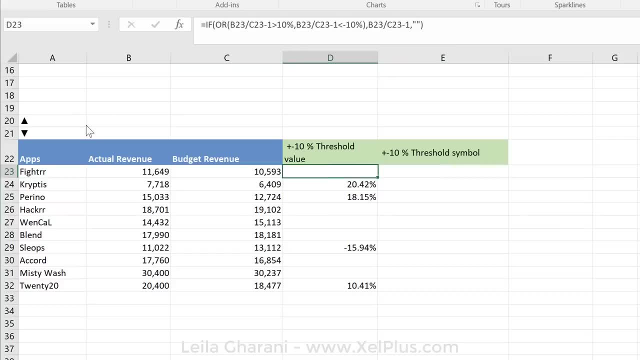 and just replace this with a symbol. I can't right Why. Because I'm using two different symbols, So I need to split them up. If I was using the same symbol, I can, but I'm not in this case. 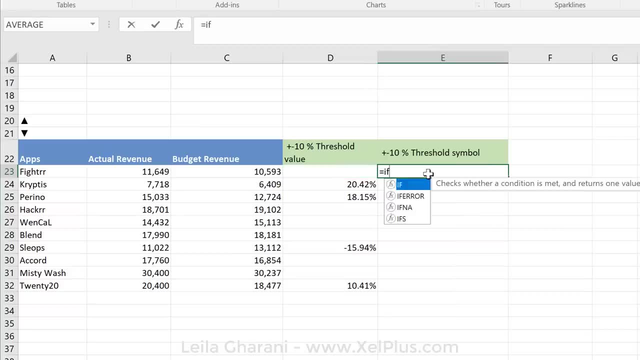 Let's just write this one from scratch. We know our logical test by now. so that's this. divided by this minus one, Let's do the positive one first. So if this is greater than 10%, then we want the symbol, which is this one: 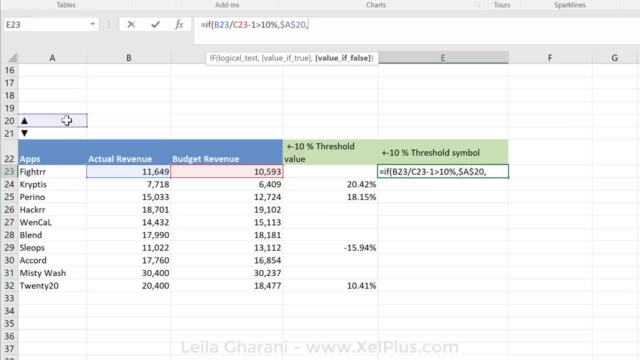 and press F4 to fix it. Otherwise, what do I need right here? Can I just put the other symbol? No, If I wanted everything else that wasn't above 10% to show this symbol, then yes, but I don't. 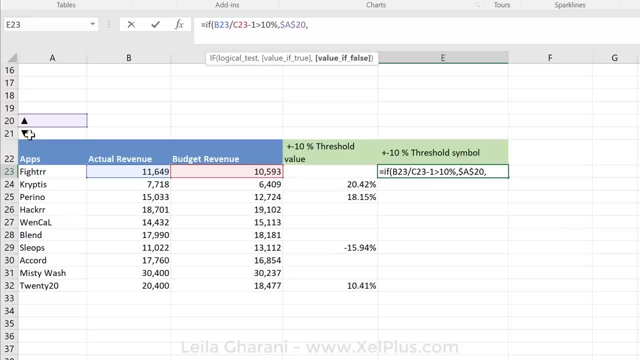 I just want the ones that are below minus 10% to show the other symbol. So I do need an if here and my logical test is the same, So I'm going to copy this and paste it in. here Is less than now. it's minus 10%.